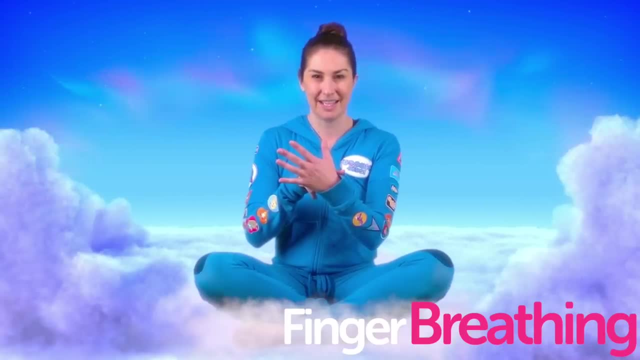 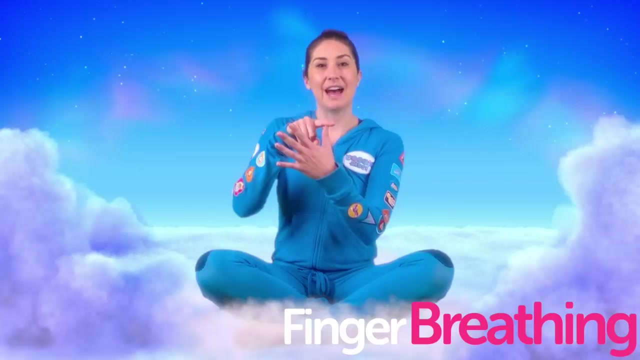 of your air. Now slowly start to breathe in and slide your finger all the way up one side of your thumb. When you get to the top of your thumb and you're full of breath, now slide down the inside of your thumb as you breathe out. Let's keep. 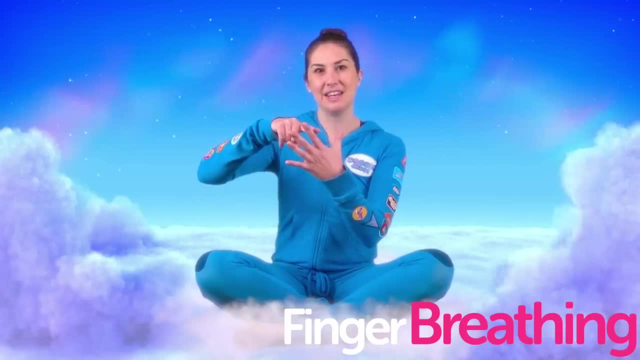 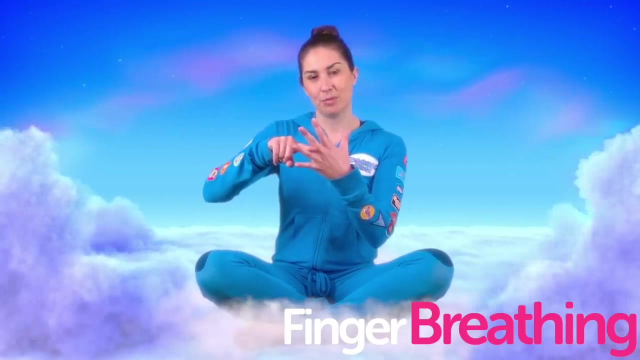 going along our hand. breathing in as we go up the side of our fingers and breathe out And breathing out as we slide down the other side. Breathing in, breathing out. Breathing in, breathing out. Breathing in and breathing out. 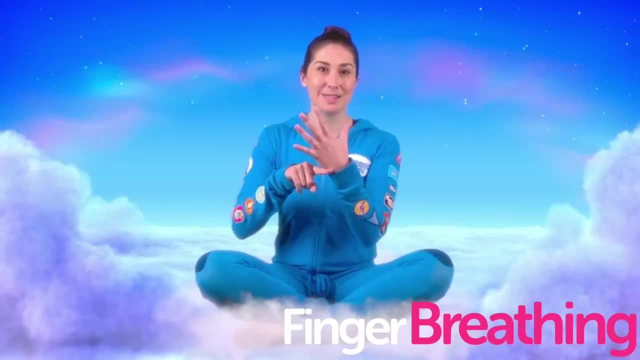 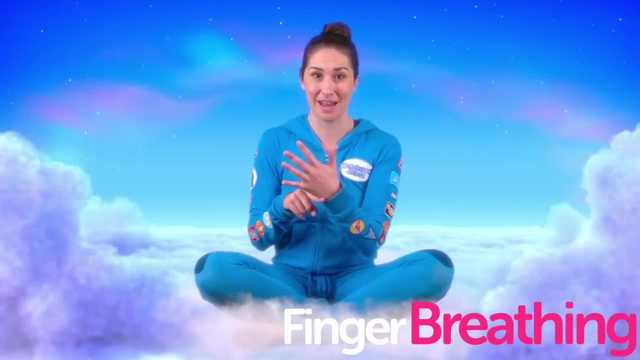 When you get to the end and your finger reaches the base of your hand, on the back of your thumb, Now take the remaining left hand and slightly push it out and keep going down your thumb. Slide your fingers back and forth between your fingers until you feel your thumb. 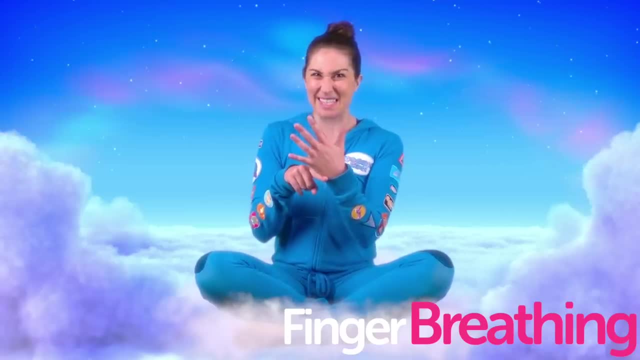 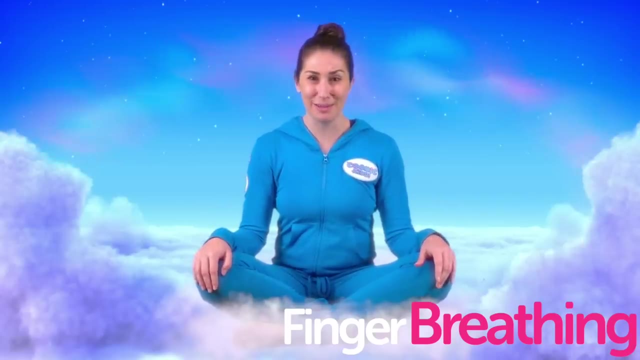 or your right olm, And when you day you feel me on your chin, you might donated your hand onto the рен of your jaw and your finger You can begin to feel something feels a little bit tender. so feel it as if you sacrifice. 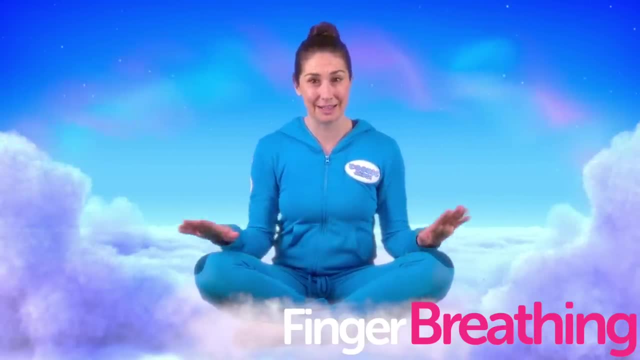 it moving back and forth. Really enjoy yourself and your hands as you are breathing. Now do another, immediately harder one, Like always. insert your finger in When you do it and calm it down. relax your fingers to the side as you breathe out. 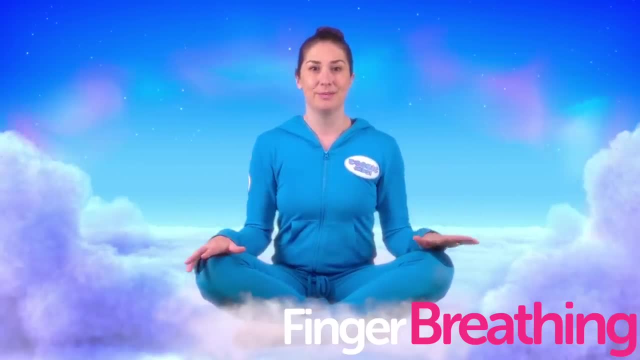 When you breathe back out, use your su walls back. Now take the other hand and dropping your fingers with your'm mound- All you. why is you tear your fingers? Now this has changed, Like I've come to make you feel calm as well. 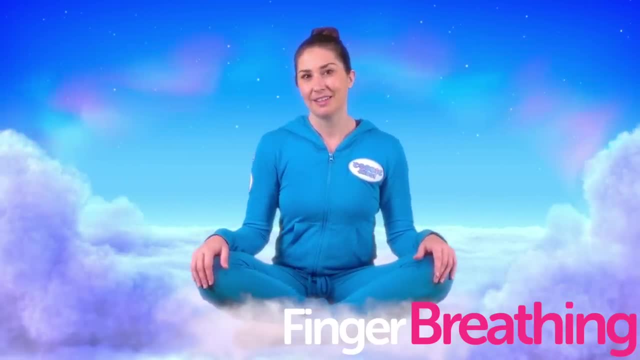 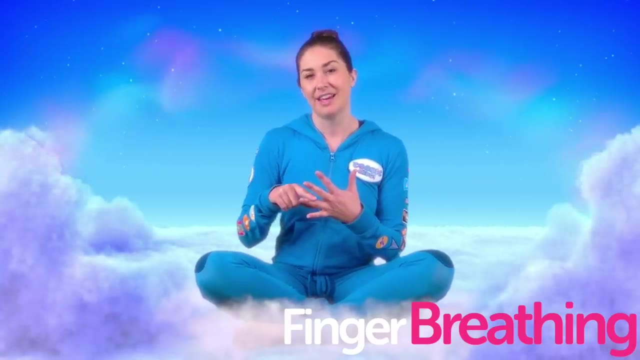 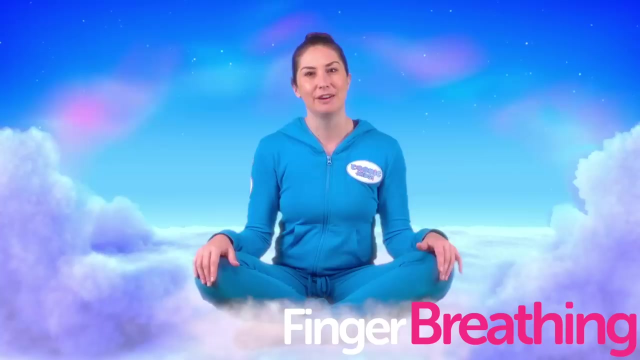 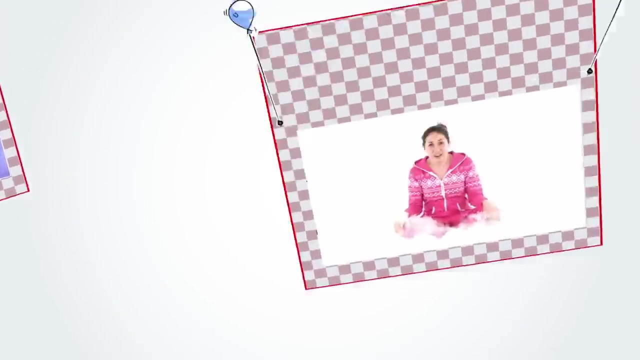 you don't even need to close your eyes, just use the outline of your thumb and fingers to guide your breath and take as many rounds as you need. it will steady you, your mind will become clearer and then you can really focus on what you are doing and do it really well. with our busy lives, we have so many things. 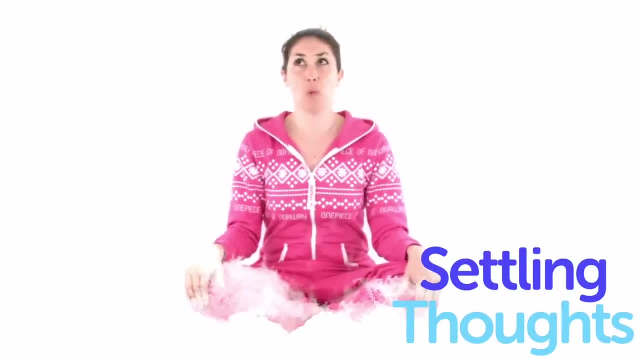 buzzing around in our heads. it can sometimes feel like a whirly-burly snowstorm. with so much going on, we get tired, we get all jumbled up and we can't think clearly. can you see all the stuff clouding up our heads, the snowflakes? I. 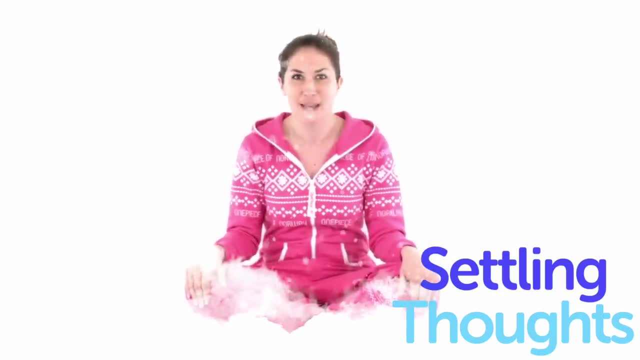 like our thoughts flying around in all directions. we need to settle the snowstorm with our secret trick: our breathing ready. let's see if we can calm this snowstorm down. we sit nice and still, can you close your eyes and tune in to all those pretty sounds? we can maybe hear some. 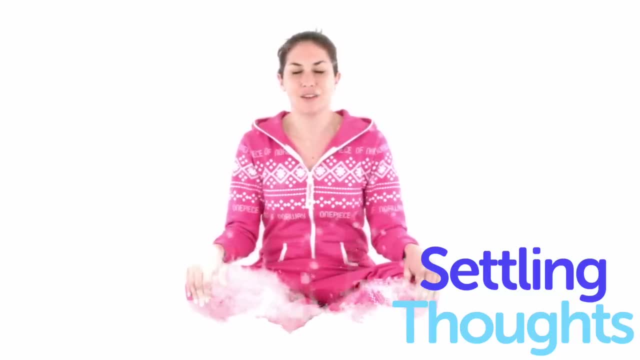 other sounds too, and if we're very quiet and we listen very carefully, we can maybe hear our own breathing. yes, we can. we can slow it right down and breathe, listening to it going all the way in and all the way out. all the way in, all the way out, that's it. 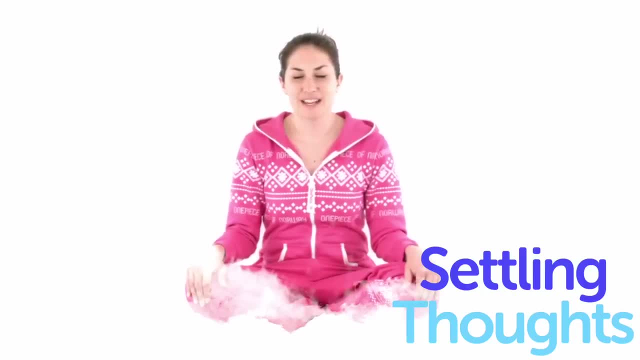 That's it. The snowstorm is starting to settle. You're doing really well. Let's keep going All the way in, All the way out. Last time, All the way in, All the way out, Opening our eyes. Well done everyone. Did you notice how calm it made you feel? 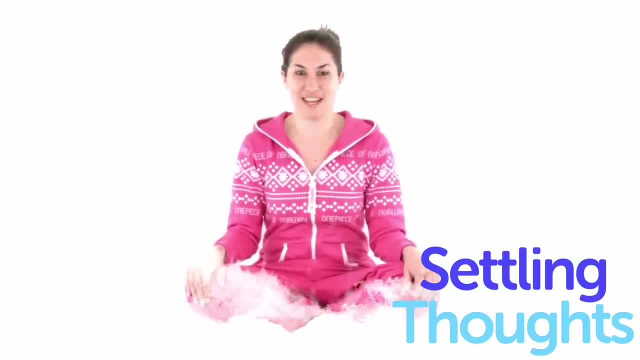 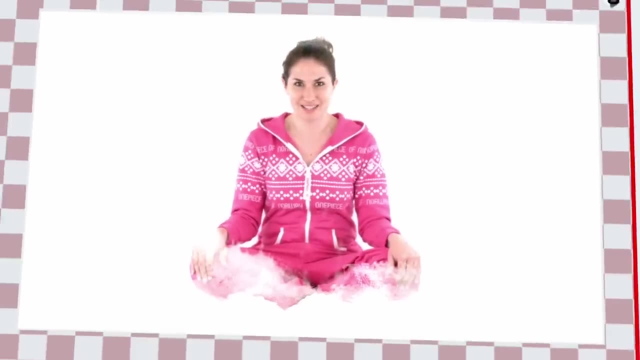 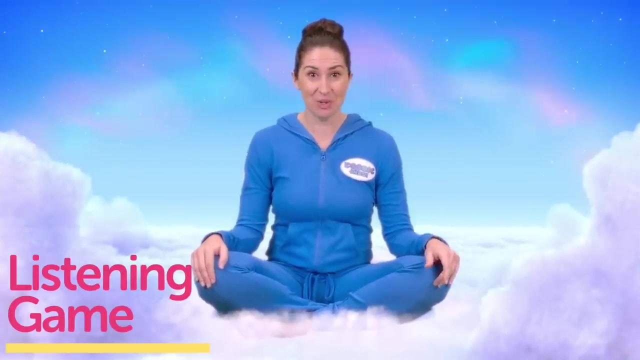 Yes, me too. All of the snowflakes, all our busy thoughts have settled, leaving a lovely, clear, fresh space in our minds so we can see our way again. Well, let's now play a special game to see how good we are at listening. 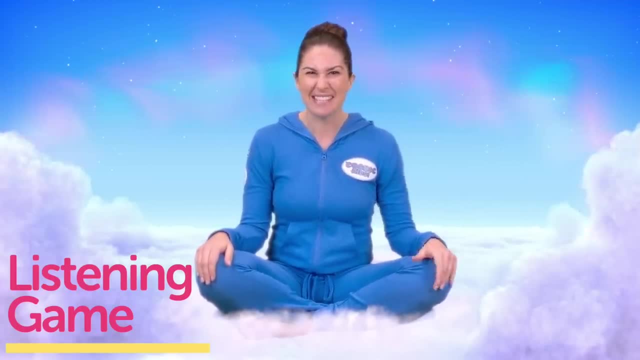 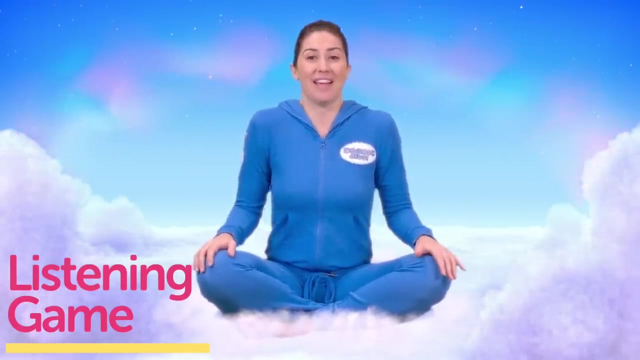 and how strong our Spidey sounds, Spidey senses are. It's time to activate our listening. So keep your hands resting on your knees, Make your back long and strong, so you are switched on and ready. Now listen, for when you hear the bell. 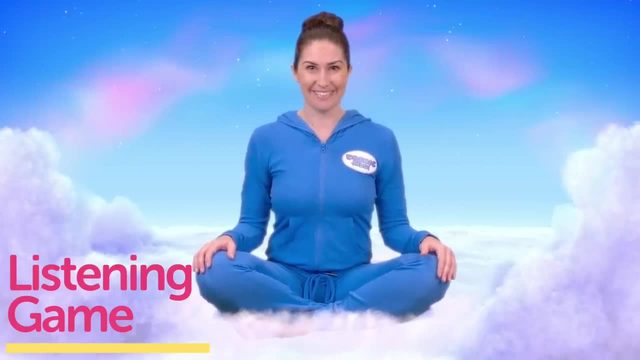 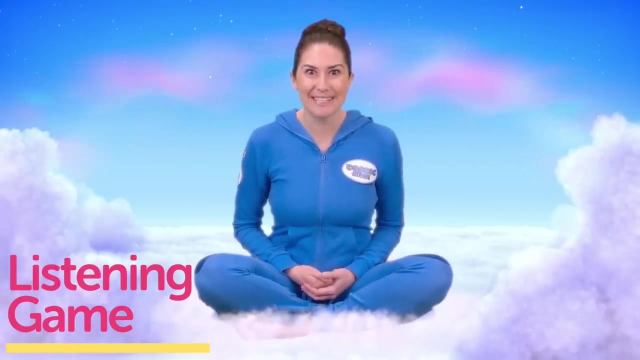 The sound will then fade until it's gone. I want to see how long you can hear the sound of the bell ringing And when you can't hear it any longer, move your hands from your knees into your lap. Then I'll be able to see how long you could hear the bell and how good your listening was. 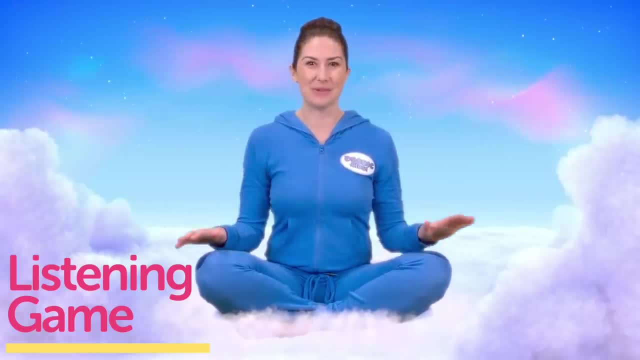 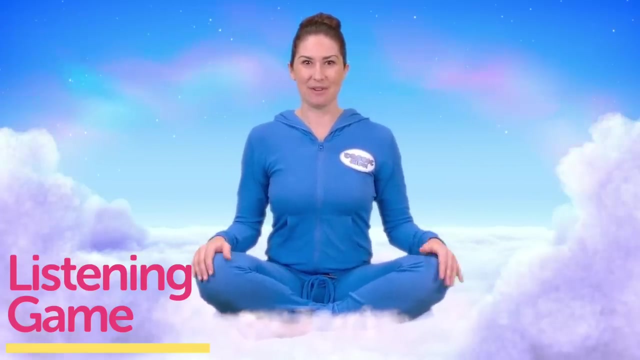 Ready, Let's take our hands onto our knees And, if you want, you can also close your eyes so you're totally focused on your listening. So here comes the sound of the bell Bell ringing. Well, that was a good start. 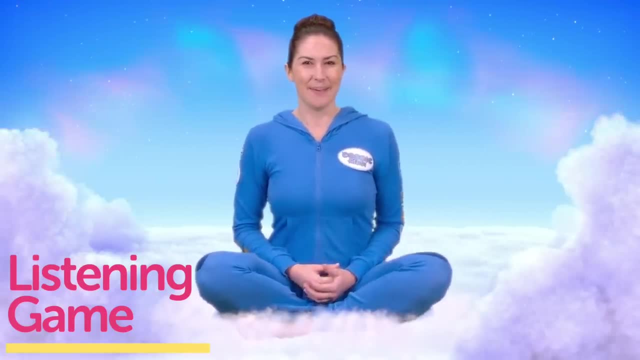 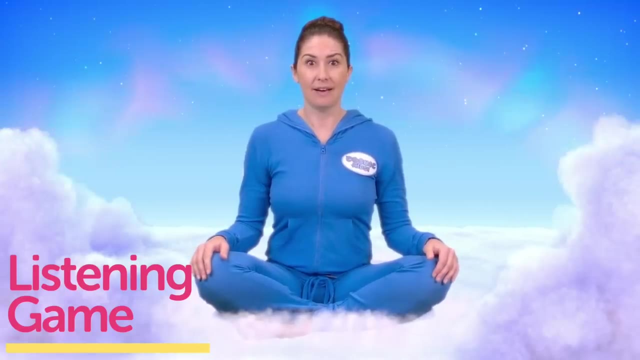 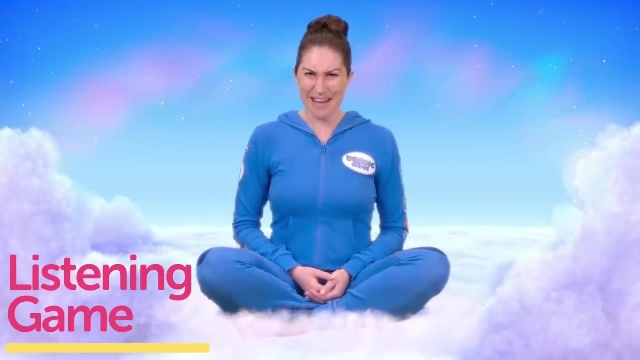 You're already showing how good you are at listening. Let's try it again. Ready Hands back to knees, Bell ringing- Cool, That was even better than the first time. Great listening everyone. Let's do one more. One last time. 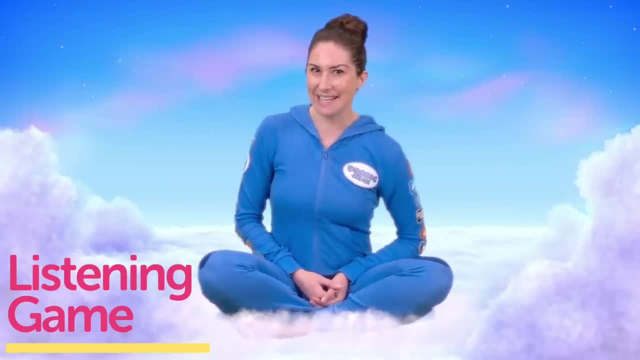 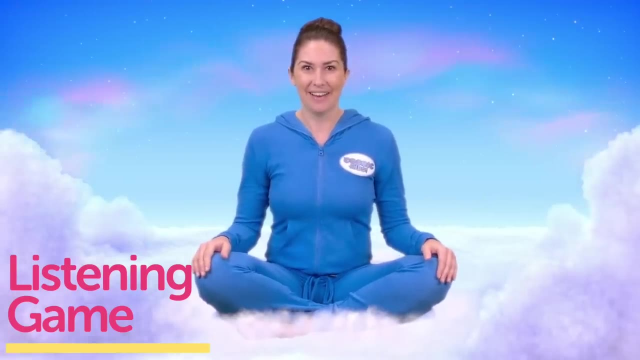 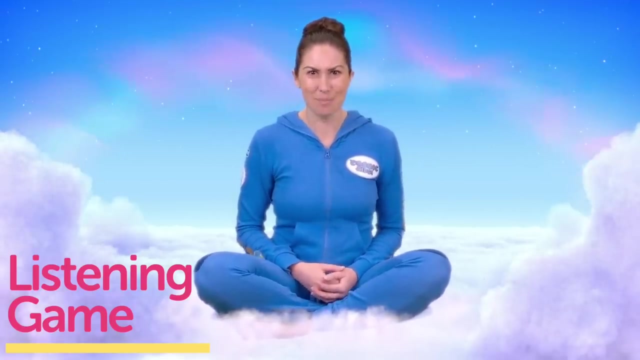 To see if we can stretch those spidey senses a little more and do our best listening. yet Ready Hands to knees And here we go, Bell ringing- Wow, That was the best one. Now you've proven just how great your listening skills can be. 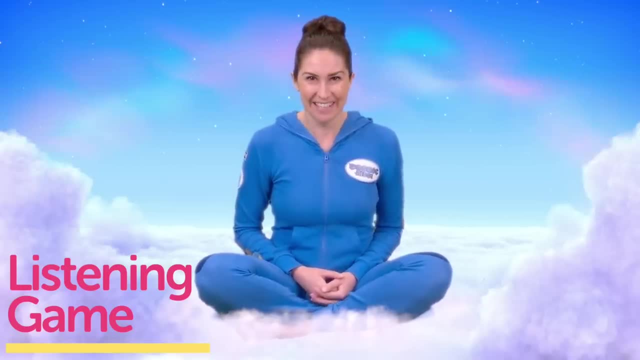 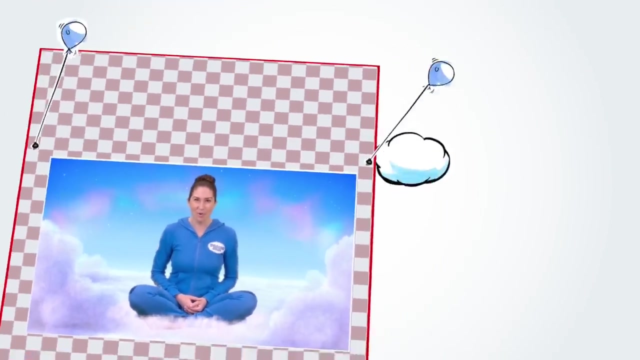 Your spider sense is activated. Next time you are trying to learn something from the teacher or someone is telling you something, see if you can activate your listening as well as you did just now in our game, And notice how much more you can hear. 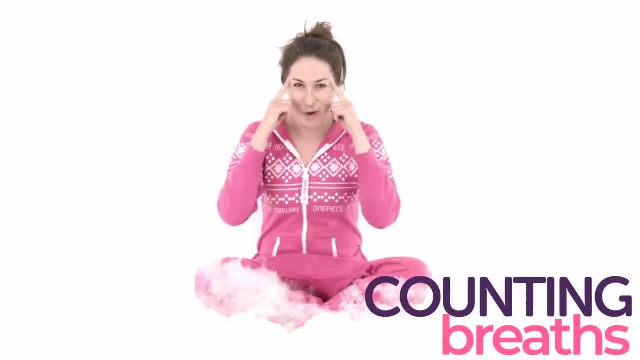 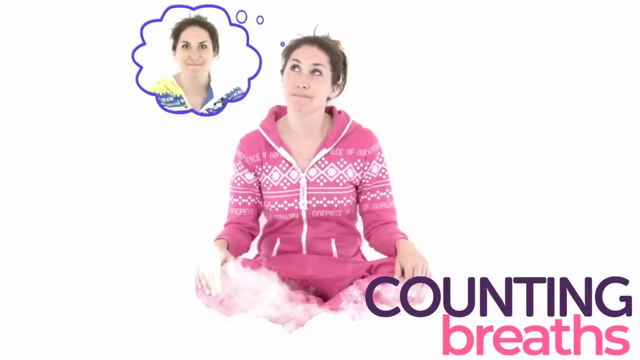 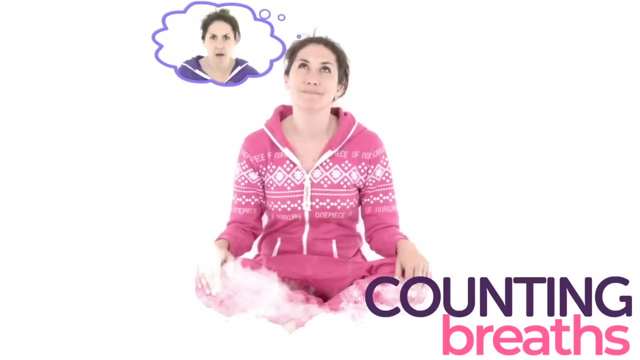 Here's the challenge. In your mind there are lots of thoughts whizzing around, Stuff like I wonder what's for dinner tonight. I'm going to a birthday party on Saturday. Where did Kira get that sticker? I want a sticker. 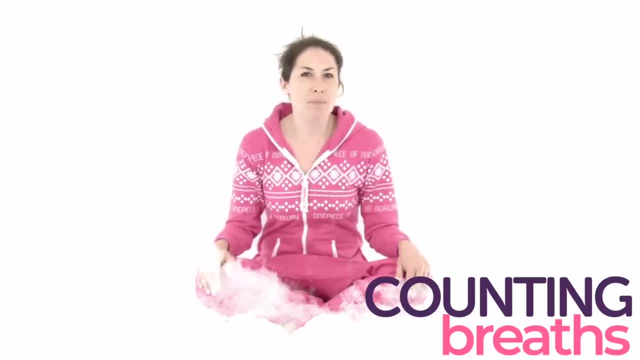 Blurgh. Our mind can be a little like a monkey, sometimes jumping all over the place from one thought to the next. It never seems to stop. There's always another thought to jump onto, And another one, And another one. If we can learn how to give our monkey mind a rest for a while, 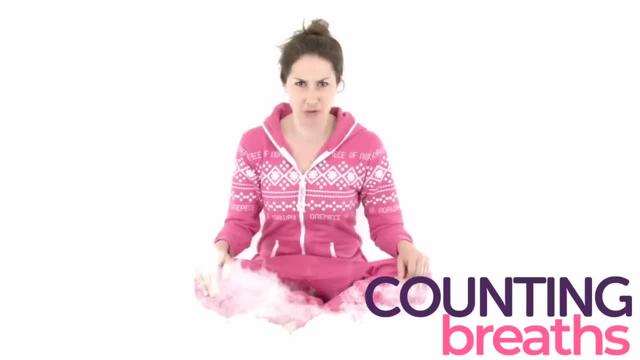 we get this superpower called concentration. To get this superpower concentration, we need to collect superpower points. Remember the breaths. For every breath you do, in and out slowly, you get one point. See how many points. See how many points you can get. 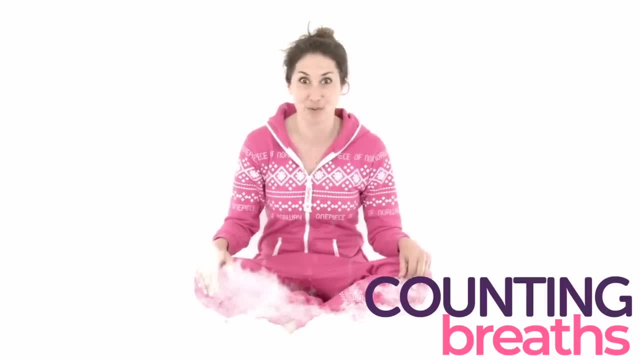 before your mind jumps like a monkey onto another thought. The secret trick is to just think about your breath as it comes in and out. See if you can keep your monkey mind on your breath and count how many full breaths you can do to get your superpower points of concentration. 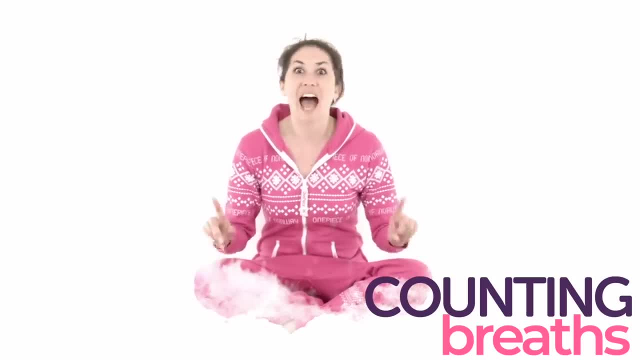 Take a moment now to do it And close your eyes too, because your monkey mind gets really jumpy and excited at all the things you see going on around you. I'll do it with you too. Ready, Let's start. See how many you can do before the bell rings. 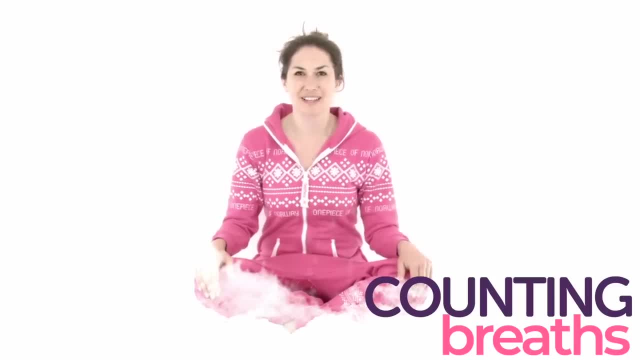 Focus on your breath, Breathing in, Breathing out, Slow and steady. If your monkey mind jumps, don't worry, Just come back to your breath. Well done, Open your eyes. everyone Now, how many did you count before your monkey mind jumped to a thought? 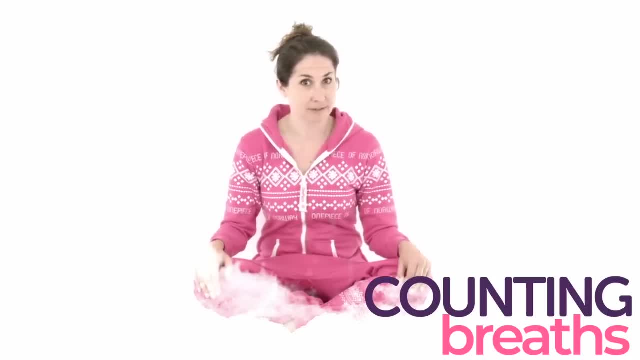 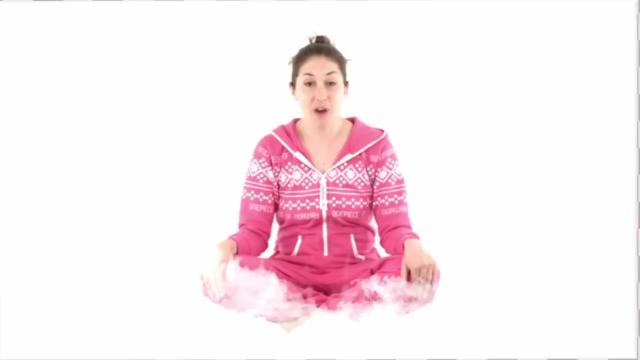 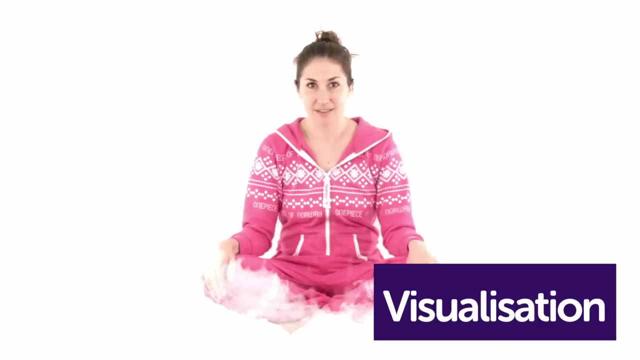 Maybe one, Ten, Twenty Or none. Be honest with yourself and know that with practice you can help your monkey mind get that superpower of concentration. Here we go. With your eyes closed, you can see a blank space, all black and dark. 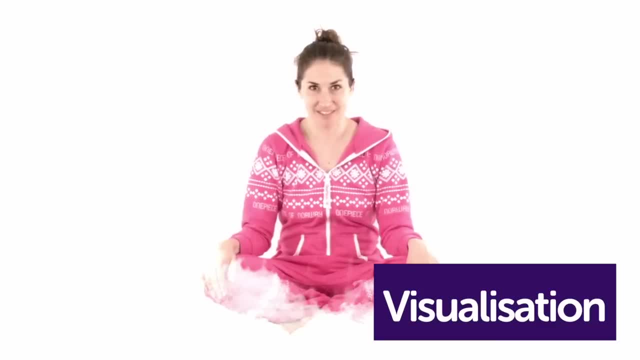 Now you see an apple, a bright green and red apple. Yes, There it is. Now you can see a red fire truck, a shiny red fire truck. Wow, Now you see a Christmas tree with its twinkling lights sparkling So pretty. 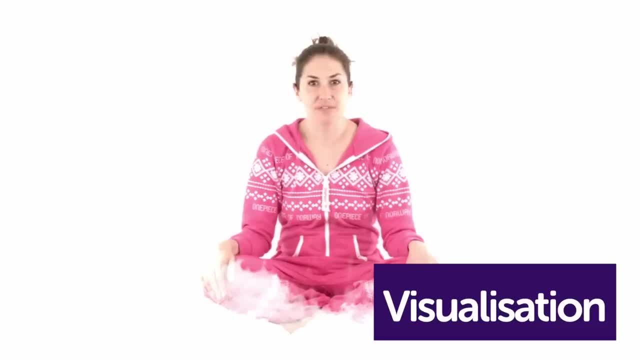 Now you see a butterfly. You can see its wings. It has the most beautiful coloured wings. Now you see a door. Looking at your door, what type of door is it? Is it a large wooden one? What colour is it? You look at your door. 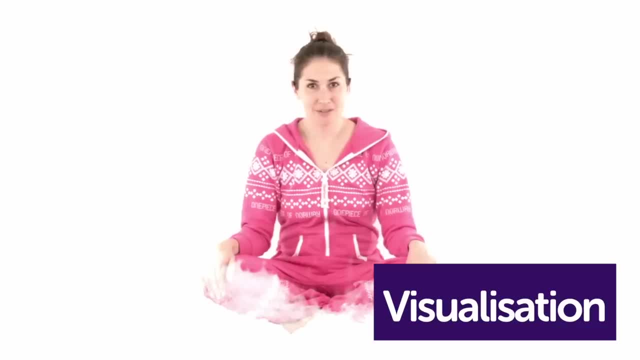 and see the handle too. You reach forward and put your hand on the handle and feel it on your hand. What does the handle feel like? You know that when you open this door, it will lead you to a place where you feel really happy and safe. 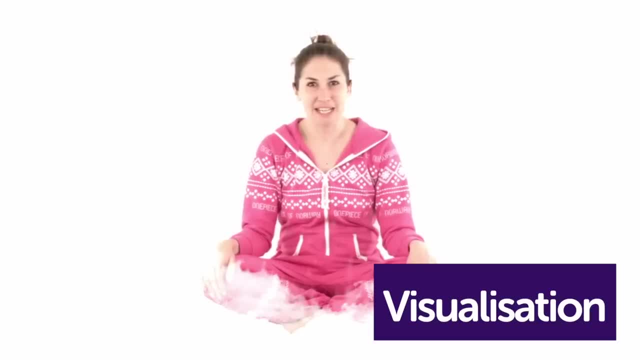 Go on, Go ahead and open it. There is your special place In the movie of your mind. what do you see? Breathe in deeply and feel what you feel. Breathe out slowly and enjoy being here in your mind movie. 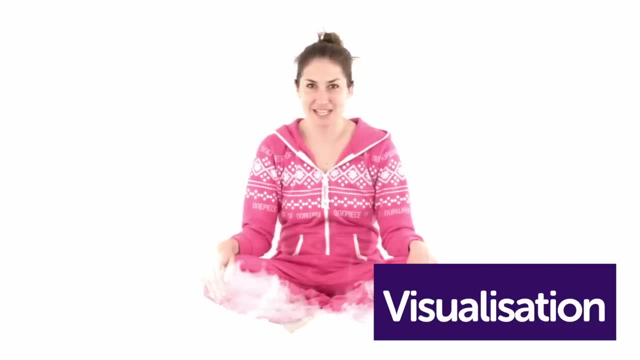 You can come back here to this place whenever you need. Now it's time to come back, to return from your little mind movie. I'll count to ten- and slowly you can come back to where you started, feeling much more calm and settled.